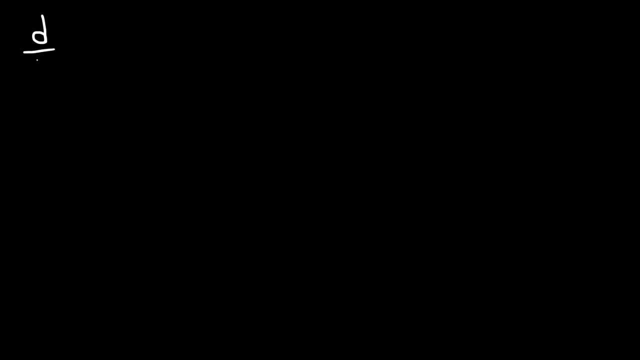 Now let's try another example. Go ahead and differentiate this expression: 5x minus 9x cubed times 8 plus x squared. Go ahead and find the derivative of this entire expression. So let's say that f of x is 5x minus 9x cubed And g is going to be the other function, a plus x squared. 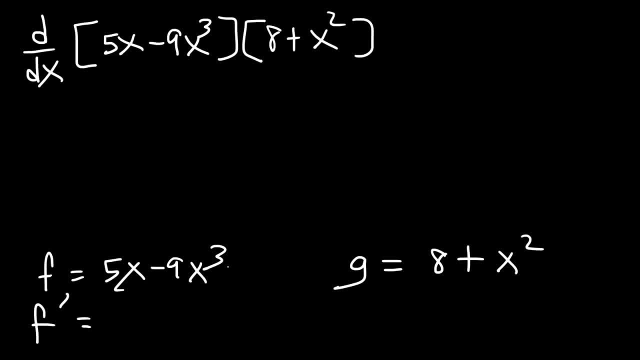 So first we need to find f prime, which is the derivative of 5x is 5, and the derivative of 9x cubed, That's going to be 9 times 3x squared, which is 27x squared. Now for g prime. The derivative of a constant is 0, and the derivative of x squared is 2x, according to the power rule. 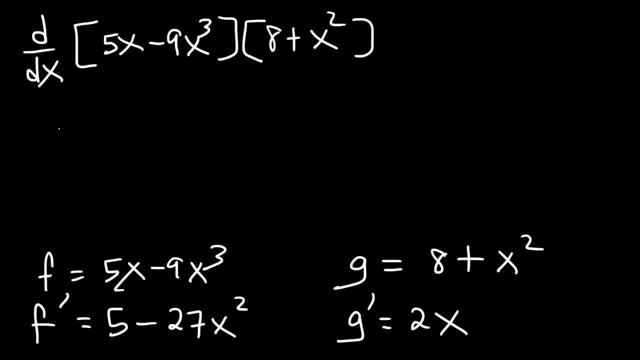 So, using the expression, the derivative of f times g So f prime is equal to the derivative of the first part, f prime times the second part plus the first part times the derivative of the second So f prime. that's 5 minus 27x squared. And g is 8 plus x squared plus f, which is 5x minus 9x cubed. 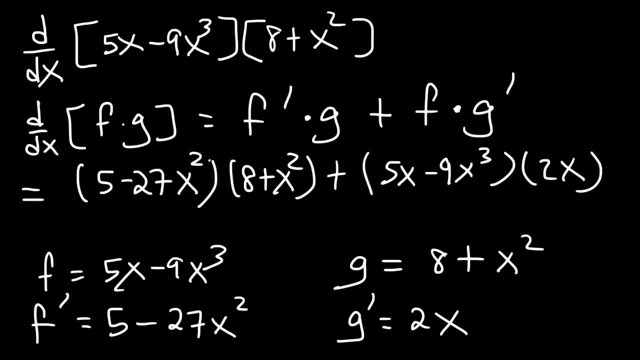 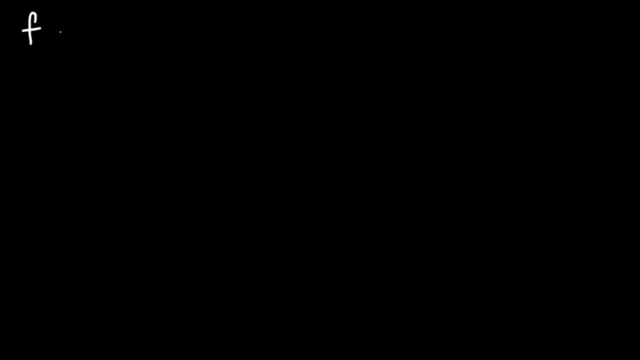 And then g prime Is 2x, And so this is the answer. Now let's try an example with trig functions. So let's say f of x is 4, sine x, tangent x. Go ahead and find the first derivative of the function. 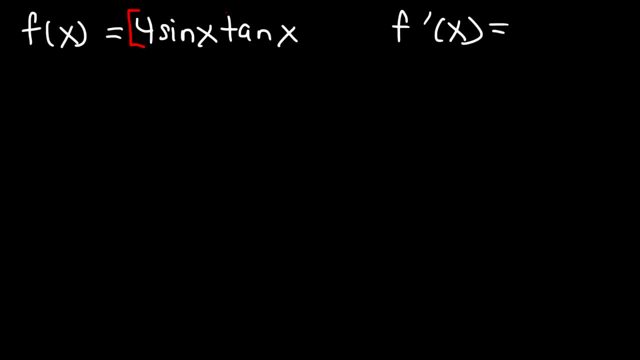 Now it's good to separate it into two parts. This is the first part, And you can call that f if you want, And then this is g, the second part. So to differentiate it, we need to find the derivative of the first part of the function. 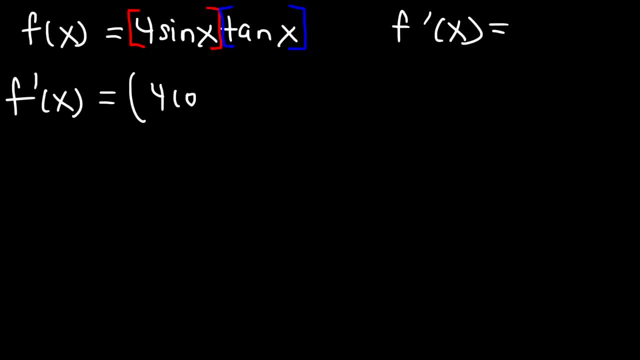 The derivative of 4 sine x is 4 cosine x. Now the second part g, we're not going to change it. And then plus, we're going to keep the first part the same, but we're going to find the derivative of the second part. 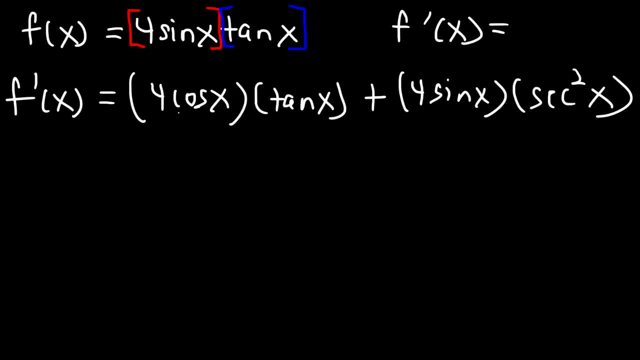 The derivative of tangent is secant squared. So, as you can see, this is f prime, This is g, This does not change. Let's say this is f and g, And then f is unchanged here, and then that's g prime. 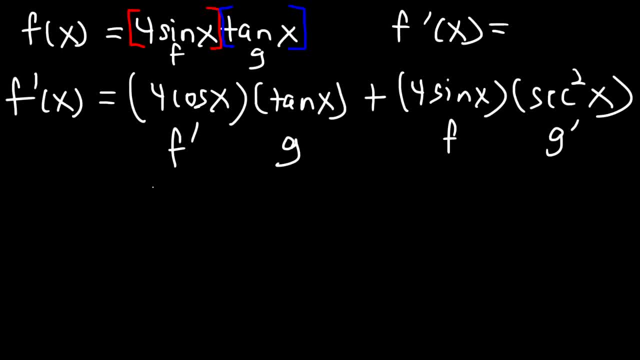 So now we need to simplify the expression. Tangent is sine divided by cosine Secant squared is 1 over cosine squared. so there's not much that we could change, But for now I'm going to just write it as 1 over cosine squared. 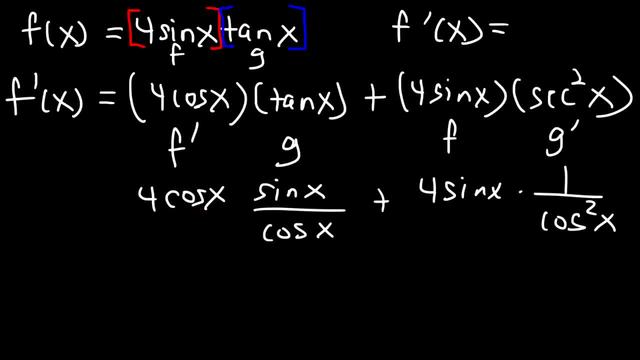 So that's the first part, And then the second part, The third part, So I can cancel cosine on the left. So I have 4 times sine x. You know what? I'm going to leave it as 4 sine x, secant squared, because I can take out a 4 sine x. 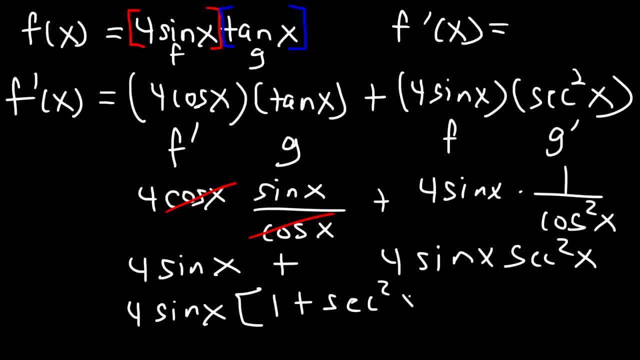 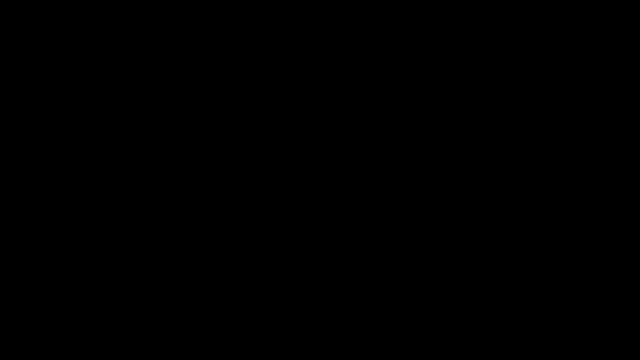 And so I'm left with 1 plus secant squared, And I'm going to stop here. So that's f prime. That's the first derivative of 4 sine x. That's 5x sine x tangent x. Now let's move on to the next example. 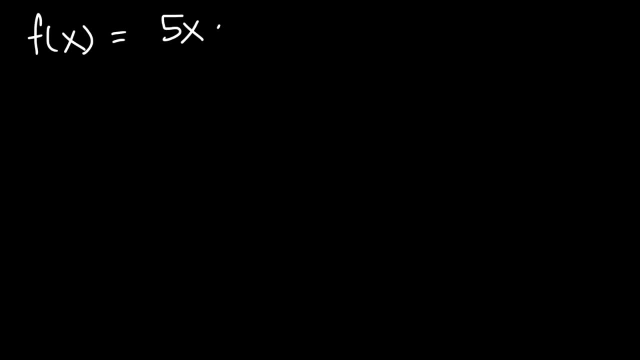 So let's say f of x is 5x sine x minus x, cubed tangent x. Go ahead and find the first derivative of this function. Now we need to use the product rule on this term and on this term separately. So for 5x sine x we can say 5x is like f. 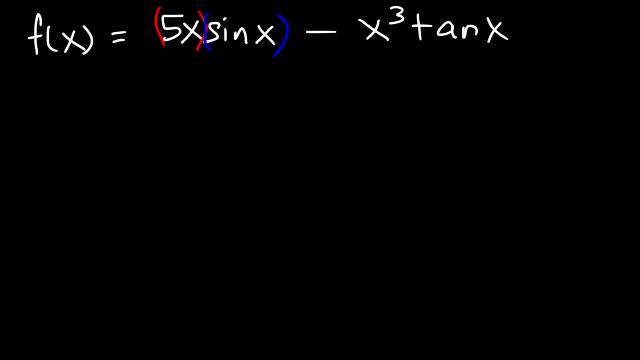 And sine x can represent g. Now for the second one. x cubed can be f and g could be tangent x. You know what? Let's call this h, so we don't confuse it with the other f. So let's determine h prime of x. 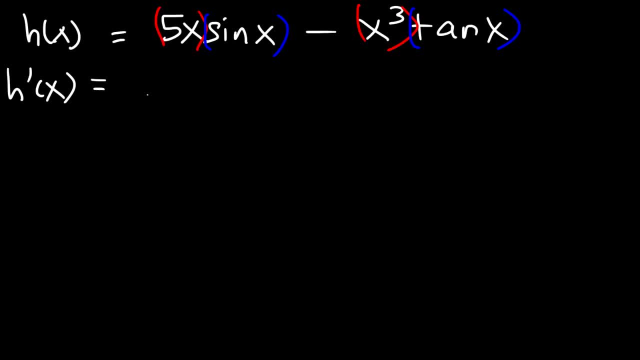 So let's differentiate the first part of the function, The derivative of 5x is 5. And then leave the second part the way it is, And then, plus, keep the first part the same. That's going to be f times g prime. 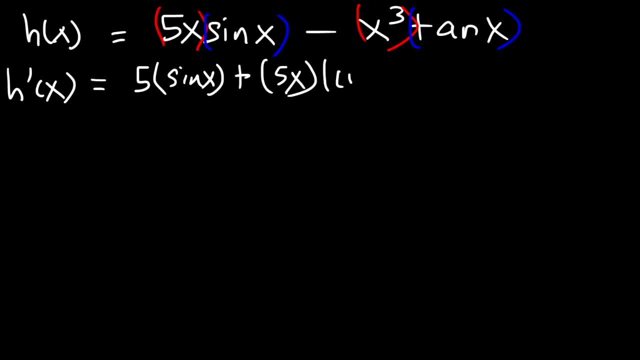 So differentiate the second part. The derivative of sine is cosine. Now let's apply the product rule to this expression, So let's enclose it in brackets. The derivative of the first part, x cubed, is 3x squared, And then leave the second part the way it is. 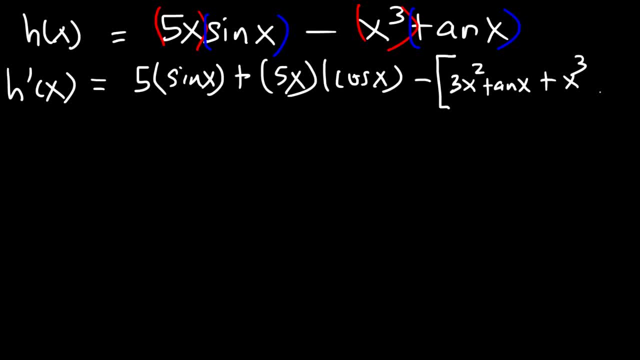 Plus, Keep the first part the same And differentiate the second part. The derivative of tangent is secant, squared, So don't forget to distribute the negative sign to everything. So we have 5 sine x plus 5x cosine x minus 3x squared tangent x plus x cubed, secant. 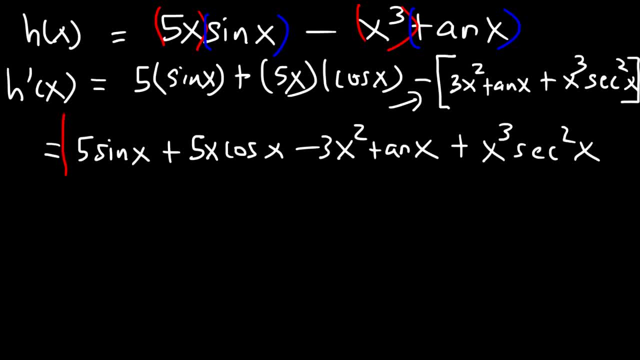 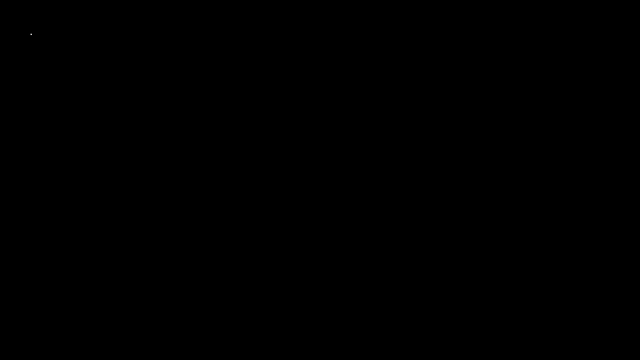 squared. Now there's nothing else that we can do with this problem, So we're going to leave it the way it is. So we're going to leave it the way it is And we will get. Oh, I almost made a mistake. This should be a negative sign. We need to distribute that negative. So this is the answer. Now let's say: if r of x is equal to x squared plus 6 times 7 minus 8x plus 3x minus 5x, 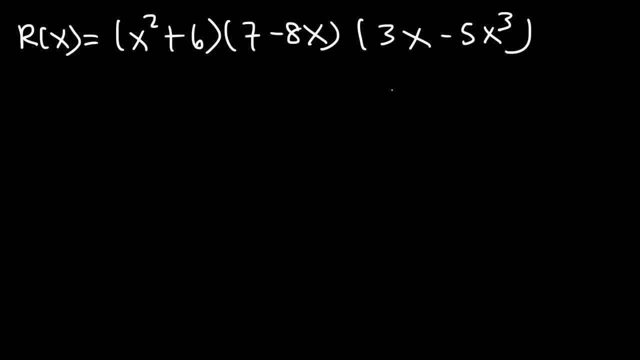 And if x equals m, if 4x, we have ceph response equal minus 3x, plus kidd- science is done- minus 5x cubed. What's our prime of x in this example? In this problem, we have three factors instead of two. So how can we use the product rule when we have three factors? We can call this: f, g. 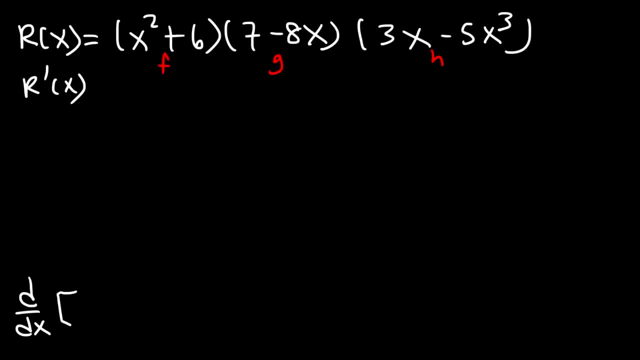 and h. So what is the derivative of f times g times h? So what you need to do is differentiate the first part, f, and leave the other two the same, and then differentiate the middle part, g, leaving f and h to the same way, and then differentiate the last part, h. So our prime: 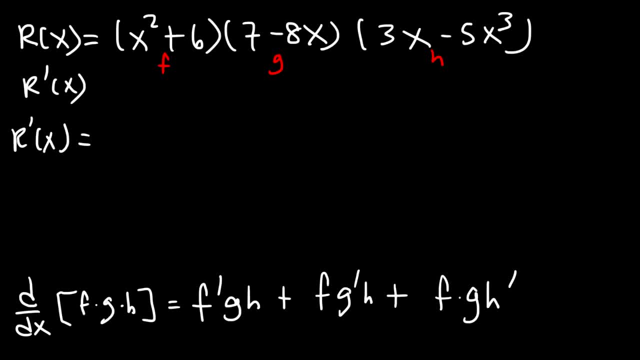 of x is going to equal the derivative of the first part. The derivative of x squared is 2x and the derivative of a constant is 0. So f prime is just 2x. And then we're going to rewrite g and h. 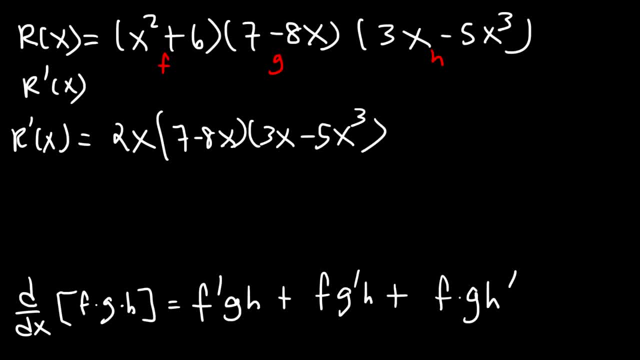 Plus, we're going to rewrite f, and then times g prime. The derivative of 7 minus 8x is simply negative 8.. And then times h, which I'm running out of space, And then plus f, which is going to stay the same, And then g is going to stay the same, Times h prime, which is going to stay the 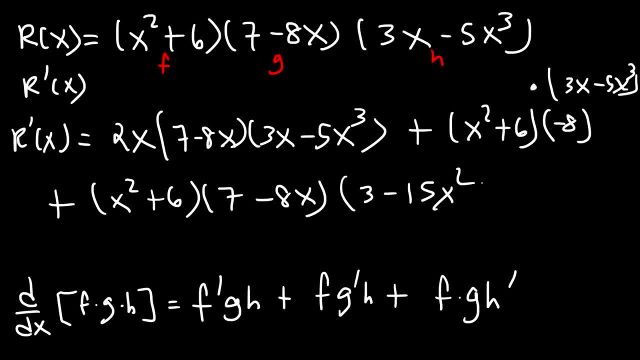 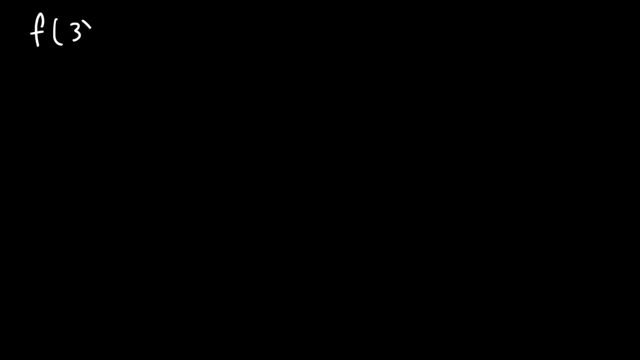 same, which is 3 minus 15x squared. So this is the answer. There's no need to simplify it at this point unless you can, But I will leave it the way it is. Now let's say if f of 3 is equal to 4,, 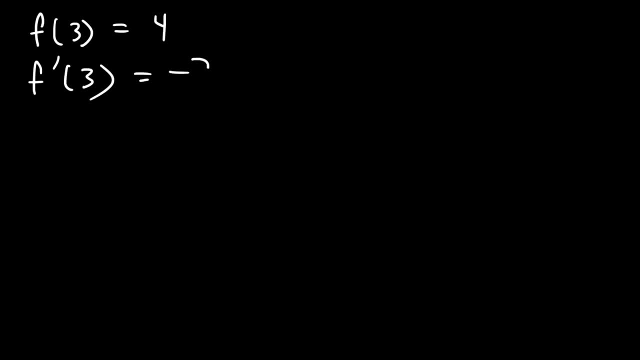 and f prime of 3 is negative 7, and g of 3 is negative 8, and g prime of 3 is 5.. What is f g prime of 3? How can we evaluate that expression? Well, we know that the derivative of f times g, that's equal to f prime g plus f g prime. 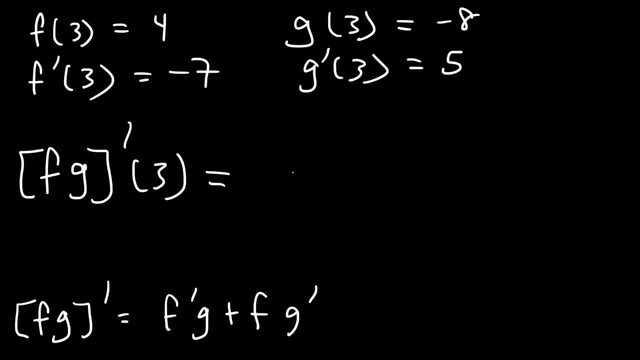 So if it's f g prime evaluated when x is 3, this is going to be f prime of 3 times g, of 3 times f, of 3 times g prime of 3.. So all we need to do is plug it into the expression on the right. 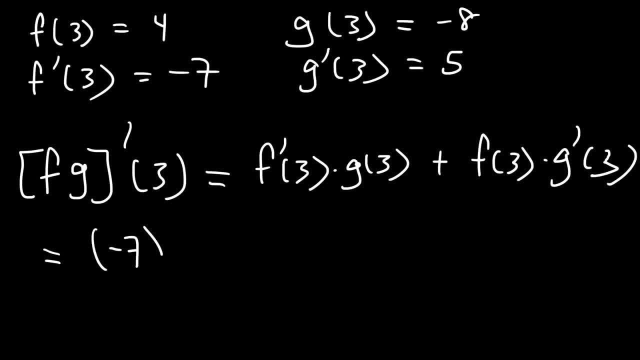 side. So f prime of 3 is negative 7, and g of 3,, that's negative 8.. f of 3 is 4, and g prime of 3 is 5.. Negative 7 times negative 8,, that's positive 56.. 4 times 5 is 20, and 56 times 5 is 50. And so 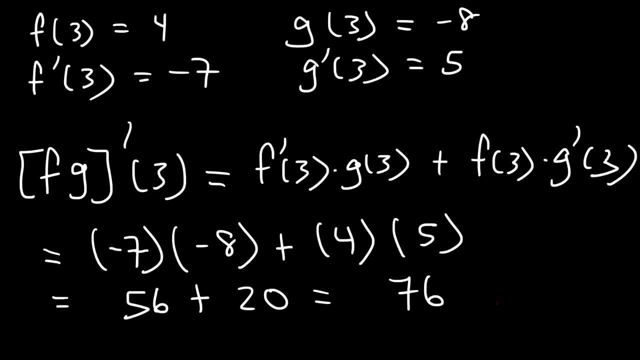 156 plus 20 is 76. And that's all you need to do in order to evaluate something that looks like this fg prime of 3.. Now you might be given this information in table form, so you can still apply the same principle to evaluate it.